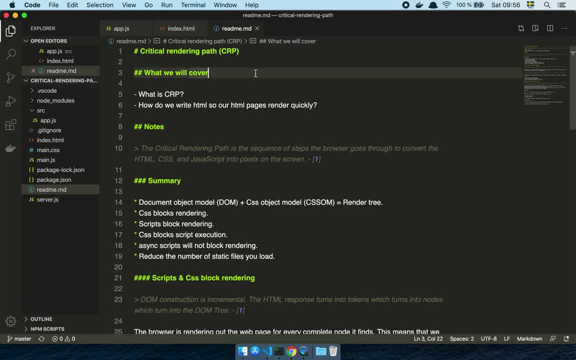 okay, guys. so in this video, we are going to talk about critical rendering path, or the critical rendering path, so let's get into it. so, crp: what we're going to cover is basically what is crp, and then we're going to go through how we should write our html in order to actually not make that. 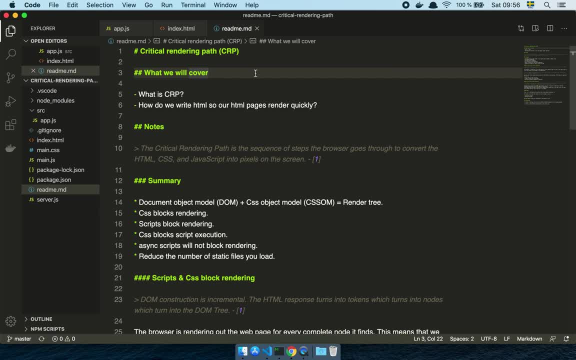 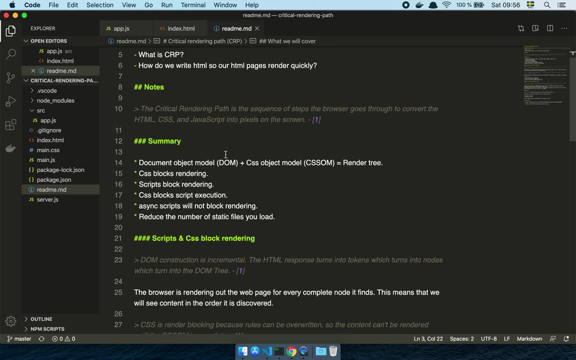 much of a problem for us when it comes to perform performance in our web applications. so i have a few definitions or quotes here from mdn, which you can go and check out later if you want to. and the first thing that we need to define is what is the critical rendering path, and it states that the 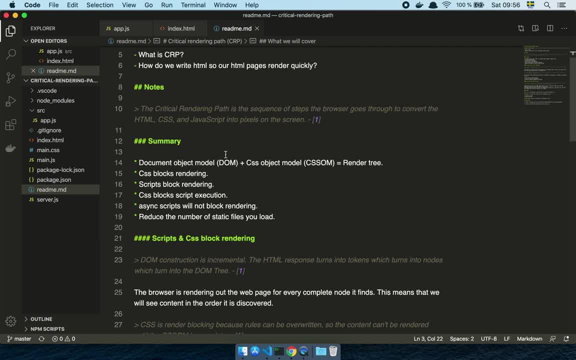 critical rendering path is the sequence of steps the browser goes through to convert the html, css and javascript into pixels on the screen. so basically, that is what's happening now. you may not be aware of this, but when you load up an html document in your browser, all the browser is. 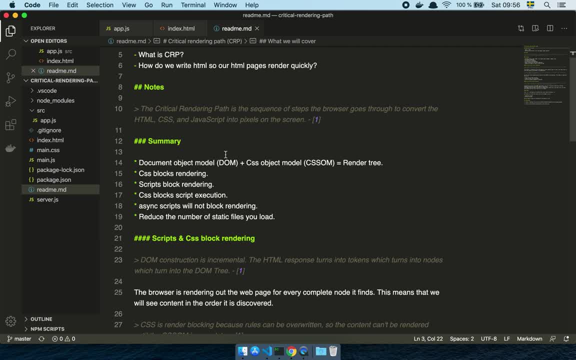 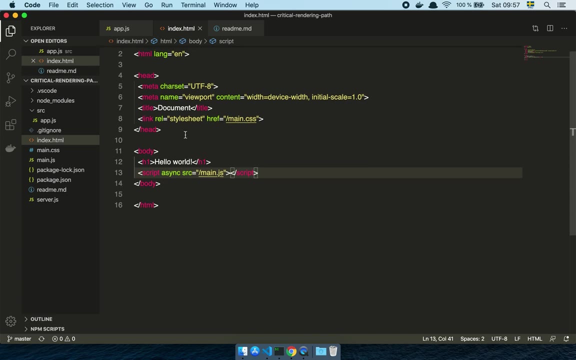 literally doing with its entire main function is to grab a html file of some sort- it can come from your local file system, it can come from the web, it can come from anywhere- and then convert the instructions or the tags. if we have a look here at our html, here, these tags is not next, not in. 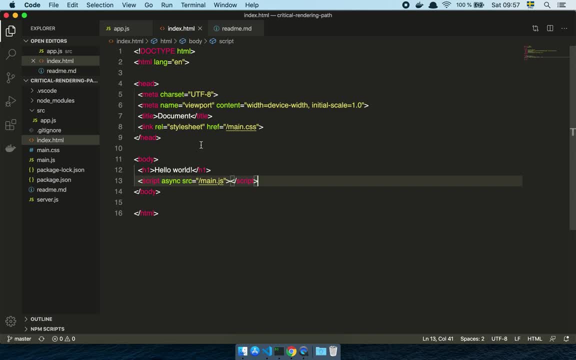 the traditional sense, will be called code, but it is code to the browser and we, the browser, will parse through all this information in order to create something that we call a render tree and then render that out into something that makes sense on the screen. so, if i 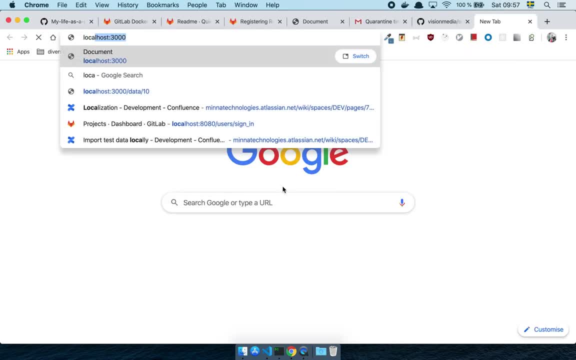 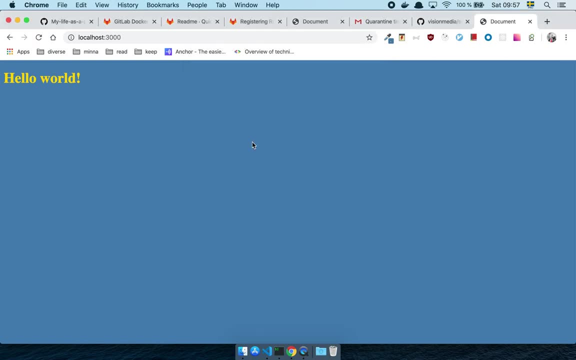 go here to my. let's see, i'm doing a lot of stuff. now let's go to my application here. so it's a alert that comes up and says hello world. and there's, this is my amazing application. what the browser just literally did was to go to localhost 3000, which is my local running server. this little. 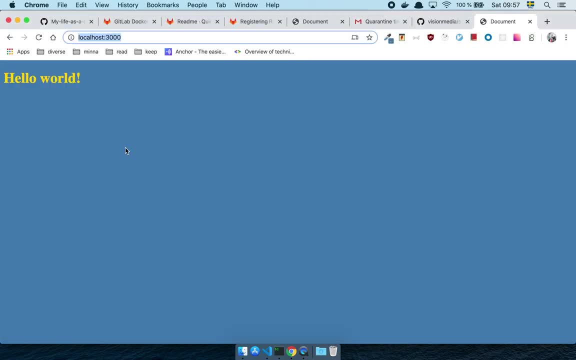 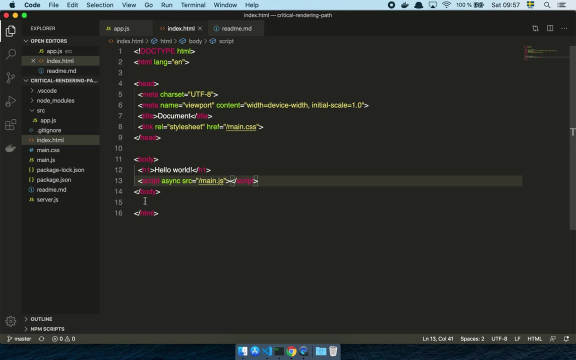 thing that i'm running right here. my little express server fetched a file in html file and then subsequently, the html file that we sent this thing here actually has a few other files. so i'm basically go- the browser is basically going through here and hitting this line here and where i've stated that. 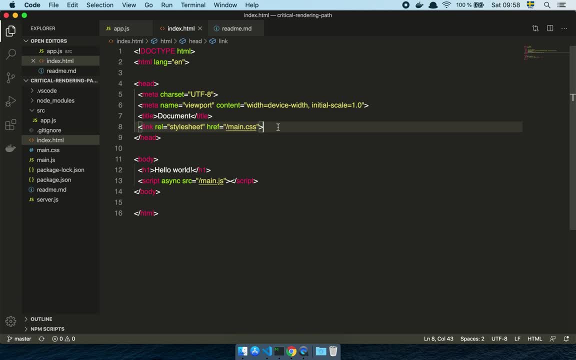 hey, you know what browser? i have another file that you're going to need in order to render out what i want to show to the user. go and fetch that file and then it's going to continue and it's going to render out the hello world message and it's going to say: oh, there's a script here and i go, yeah, go. 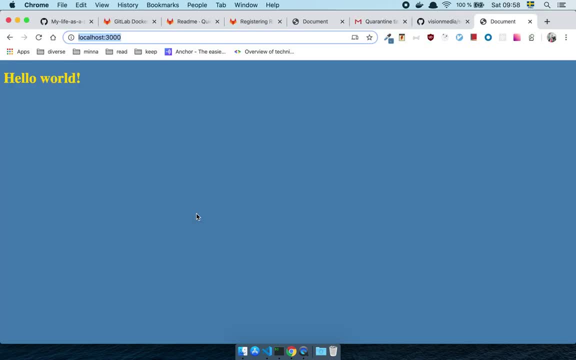 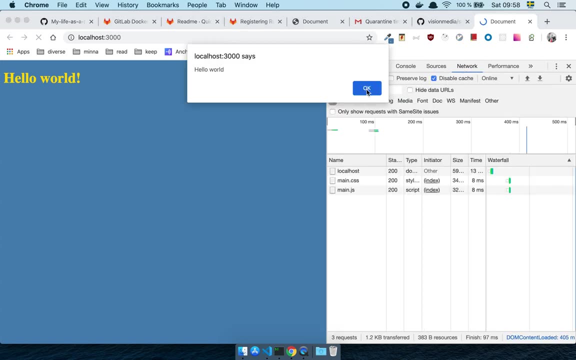 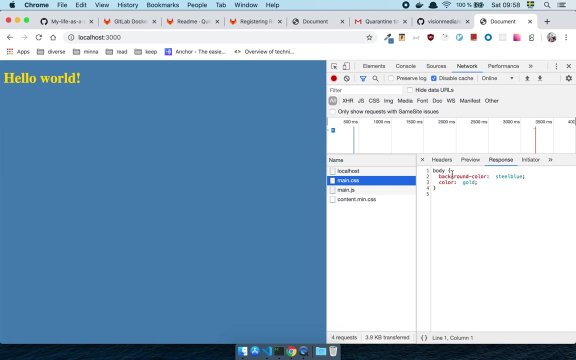 and fetch that as well. so that is in essence what's happening, and if we have a look here at my network tab, if i refresh this page, you will see that that is exactly what's going on. so here is my html file in the preview hello world, and then here is my main js with my styles. so if you look at these things in isolation, 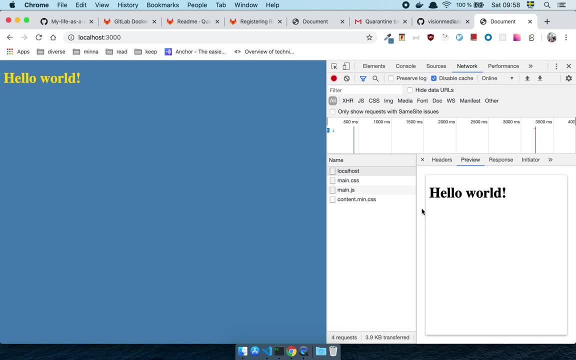 this is what the file is look like, what my html file looks like, without any of the other files, and then, with the css, i'm going to apply the background color and the text color and then, finally, i have my little javascript that is going to run the hello world alert. that's it. 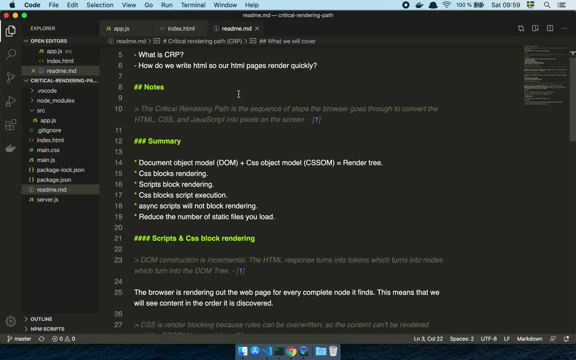 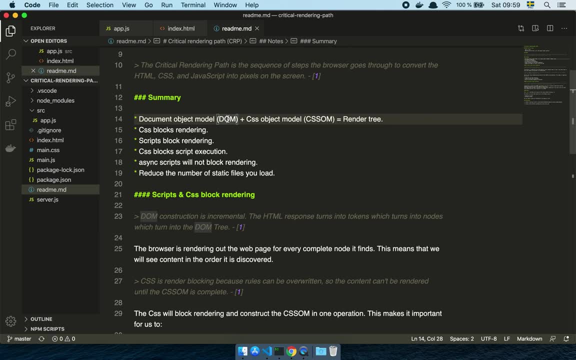 so this is, in essence, what's going on when we're talking about the critical rendering path, or crp. so i want you to make- i want to make this super clear: there's two things that are needed in order to create the render tree, which is the thing that is literally going to render out the layout. 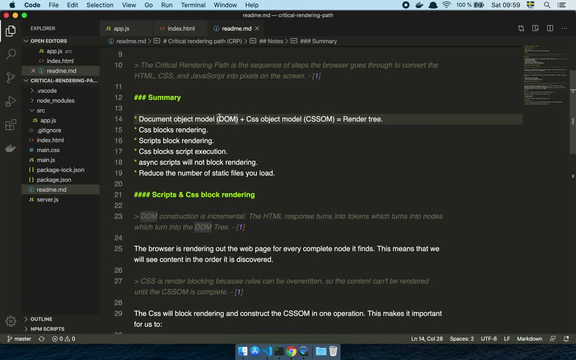 or basically to make something appear on your screen, the dom which stands for document object. this is the thing that the browser is building when it's going through the tags. now you may think that the browser is going to parse this entire file and then render thing everything. 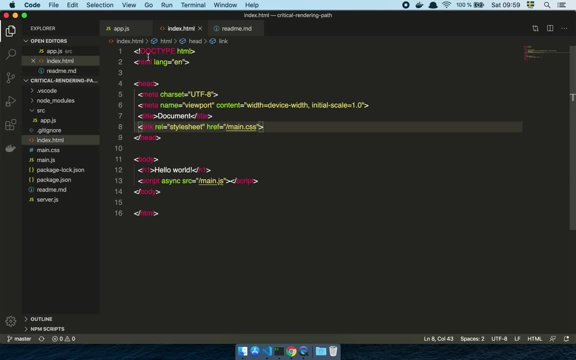 out. that's actually not what's going to happen, and you're going to see that in just a moment. it actually parses and renders as it goes along until it hits what we call a blocking call or blocking operation, which is going to be this css link here and this script tag here. well, 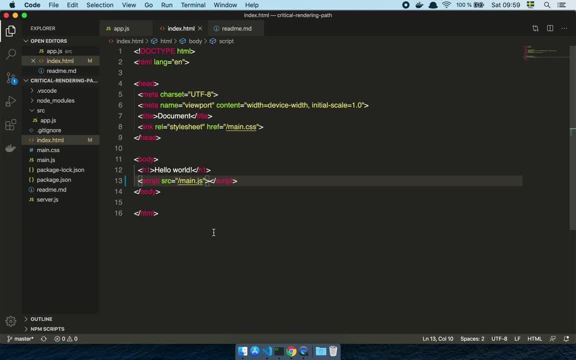 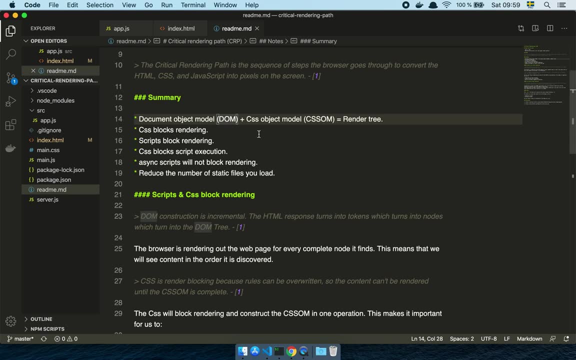 not technically, since i have a sync here, but if i do that, then this is going to be considered a blocking operation. we'll touch on that in just a moment. so that second thing that needs to happen is that we need to have the css object model or css om, which is, as you probably have guessed, it is the css. 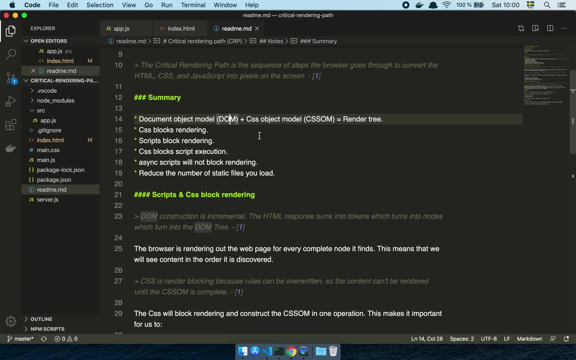 object model that is required in order to do the styling of the page. i hope that, to make that super clear, there's two. there's two object module models. you have the document object model and you have the css object model and that creates our render tree that is then used in. 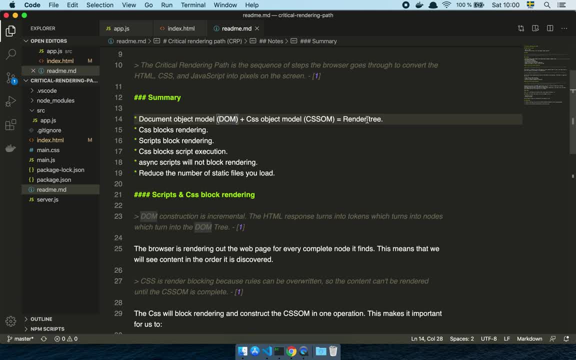 order to lay out something on the page, which is the last step, where we basically create a layout that just checks the dimensions of your screen and then it paints all of the pixels to the screen. so, with that said, there are a few things that we need to touch on here. so, as i was saying, there are 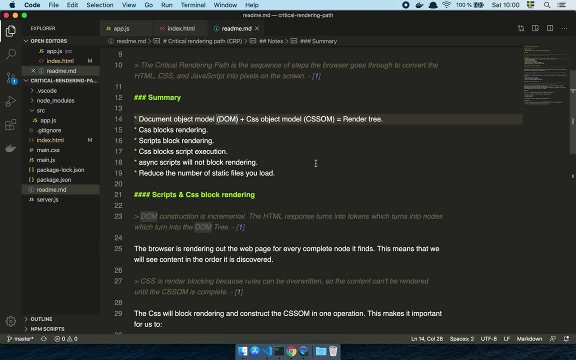 things that we call a blocking operation, and these are the things that we need to be aware of if we're going to create a page that renders fairly quickly, right. so the first thing is going to be to that you need to know that css is a block. it's go, it's going to be a block and it's going to. 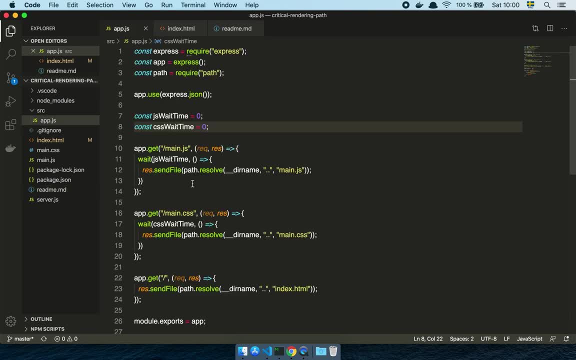 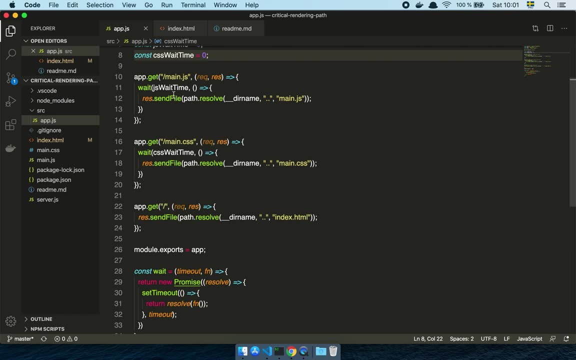 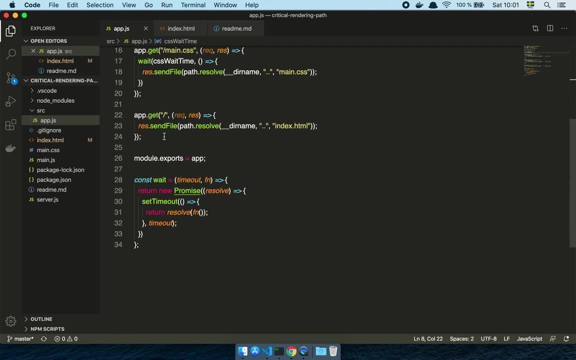 block rendering. i'll show you how demo this through this little application that i made. so here is my little simple express server, and here you can see that i have two endpoints. the way i can, i'm going to get my main js file and one that i go i'm going to get my css file and here is. 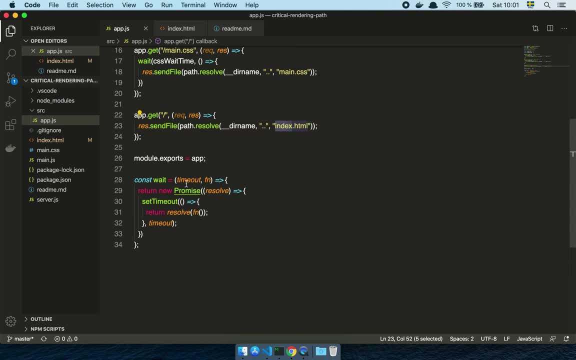 the page where i actually am getting the index html file that we saw, and then i have this little function that i created, which is just the what i call a weight function. all it's going to do is return a promise and it's going to resolve that promise after the and initialize a timeout, which. 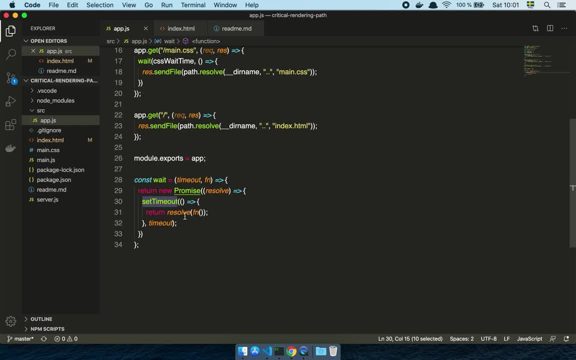 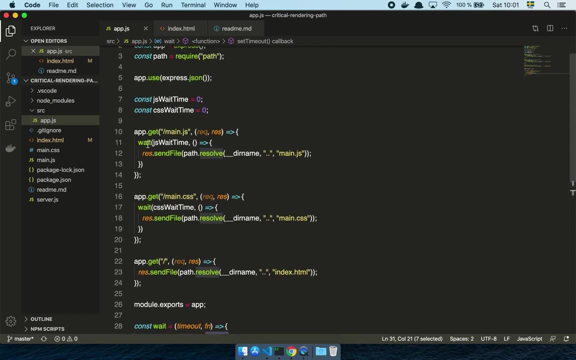 is just a way for me to wait within javascript and then, when the timeout is done, it's going to invoke this function as part of the resolution, which allows me to do this. i can wait and just delay the response that the server is going to send back to the browser. so if i now do something, 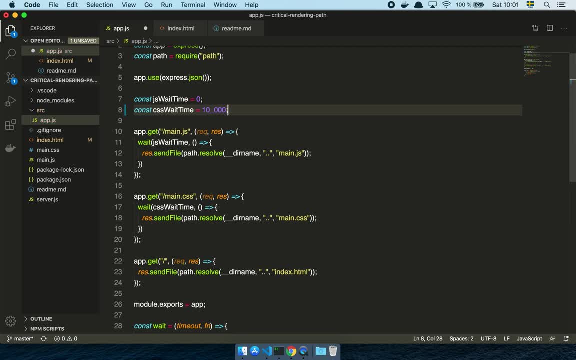 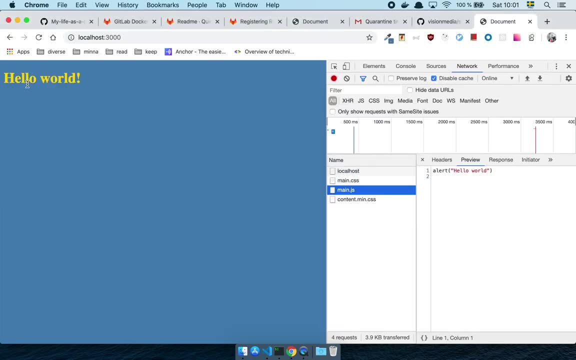 like this. i do something like this, i say ten thousand milliseconds or ten seconds for my css. notice that when i loaded this earlier, i actually saw this label here over the hello world part very quickly. so let's see what happens if i do this. so now i'm refreshing. now, yeah, i'm seeing. 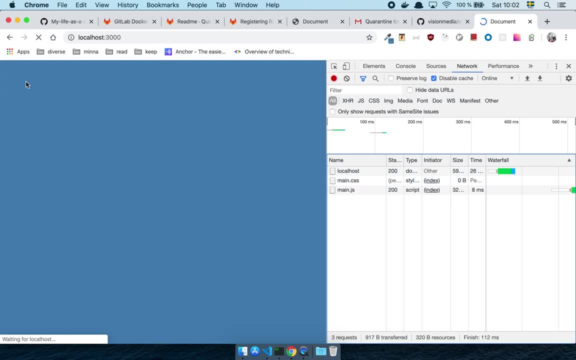 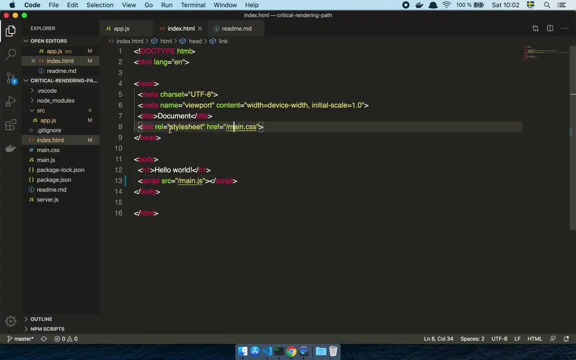 like: yeah, exactly so the browser took a moment here to remove the caching. but you see that i'm not actually seeing anything until i actually get the response back from the server, because what's actually happening is that the browser is hitting this line here and so i'm saying, all right, uh, i'm gonna have to wait with rendering out the rest of this. 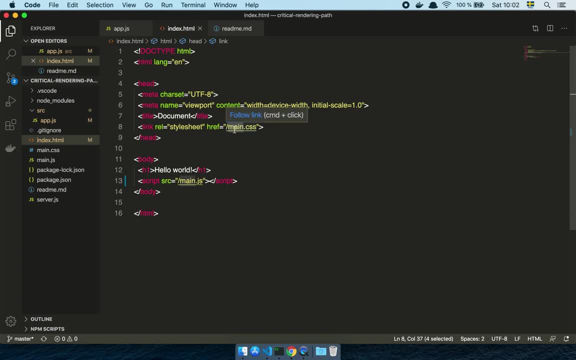 until i get back this file, because it's not safe for me to continue. or rather, the way that css, the css object module, works, is that whenever you're requiring css, it has a different behavior from the document or the, the document object model or the dom css, the css object model, is going to. 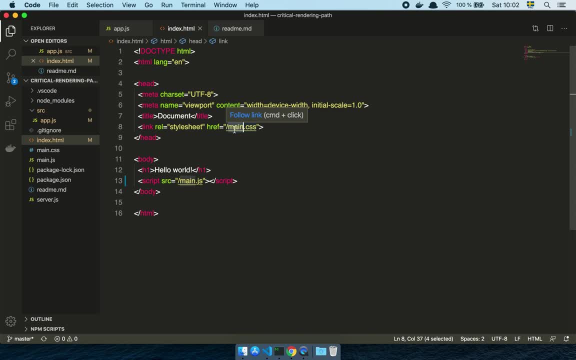 be compiled instantaneously as one single atomic opera or as one operation, and this is what this is doing. this is why it's not allowing you to continue, because it needs to compile all of the css in one go here, and the reason for that is basically because the in order 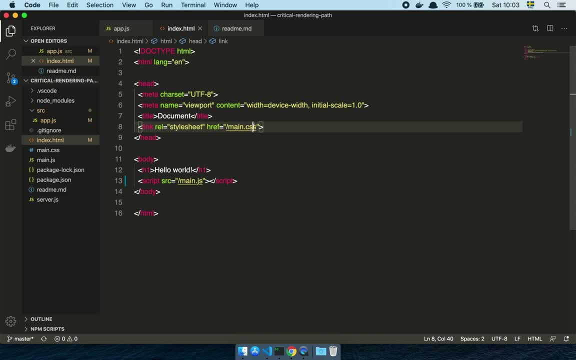 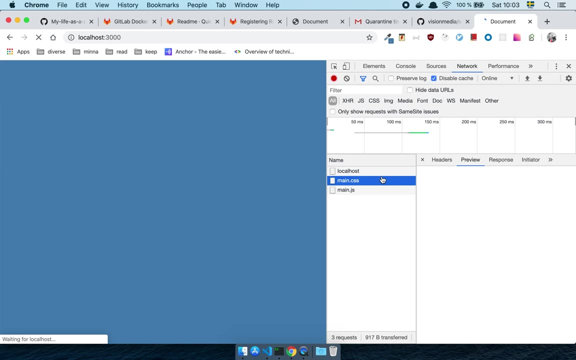 for two. for you to be able to render out the entire document, you need to have the styling and the styling needs to be be in place before you're actually done with the entire rendering. so that's pretty much. it really like the. as you can see, it's just blocking this thing, but i already 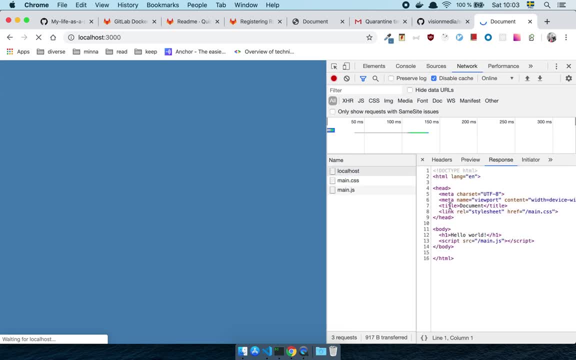 have my html, so this has already arrived at the browser. this is, but this thing is taking a long time. so the first learning that we should have from this is that the it doesn't matter how quickly we send the html. if there is a really slow network call from my css, it doesn't matter that. all of this. 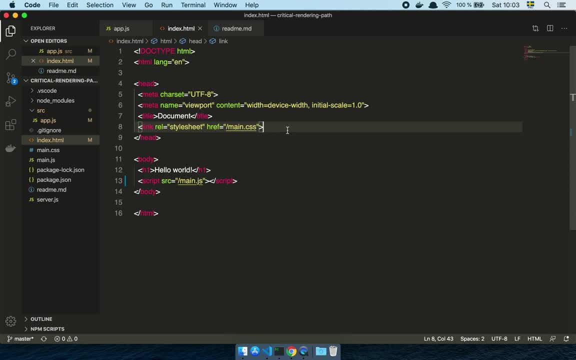 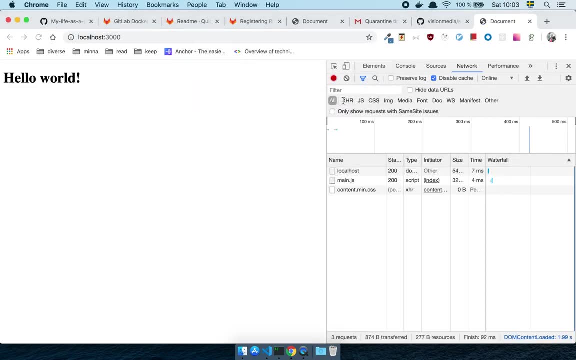 information is already in the browser, because we can't see anything on the page until this thing is done. the second: i remove this call: everything's gonna. i mean, i'm not gonna have any styles, but everything is going to be there very, very quickly. so if you want to have the fastest possible paint time or first render time, which 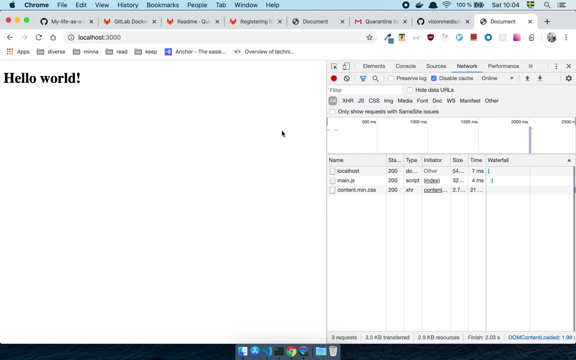 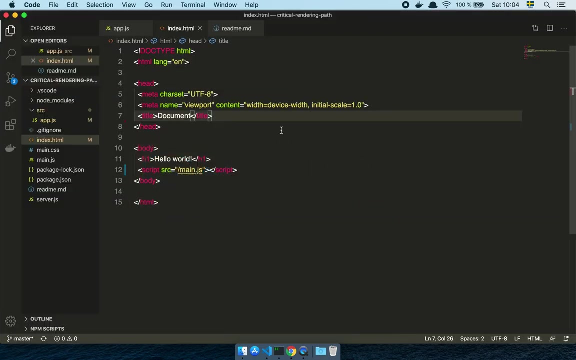 is the thing that we use cpr for. you can see rp. i mean, then, having no css is a good thing, or, at the very least, make sure that you don't have that much css, or you can inline your styles within the html, things like that- to get this thing to go as quickly as possible. now, of course, in a realistic 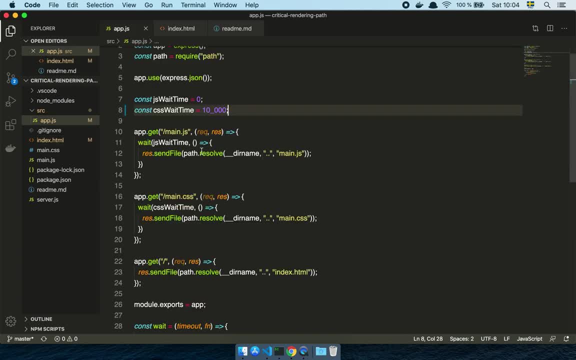 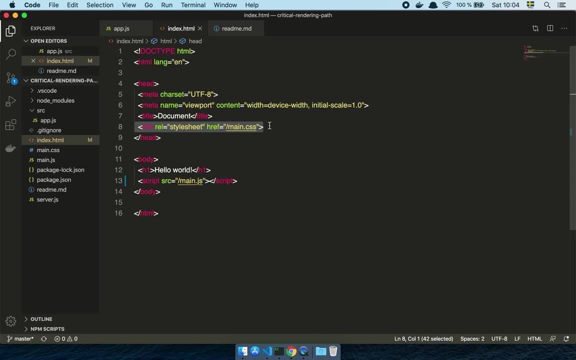 situation. you're not going to have to wait for 10 seconds to get you to get your css, but i hope you's you're on. you understand what i'm saying here. another aspect to consider here is that if you have something like this now, you're starting to have another sort of problem where every remember 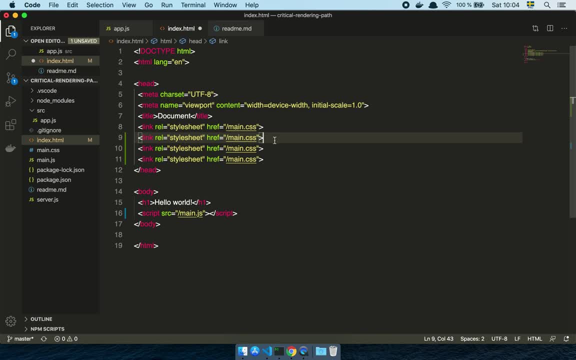 it's going to stop here, get this file, and then it's going to get this file and it's going to get this file and so forth and so forth. so if you're adding css style sheets to your document, try to add it to one single document, if it's possible. the fewer network requests that you do. 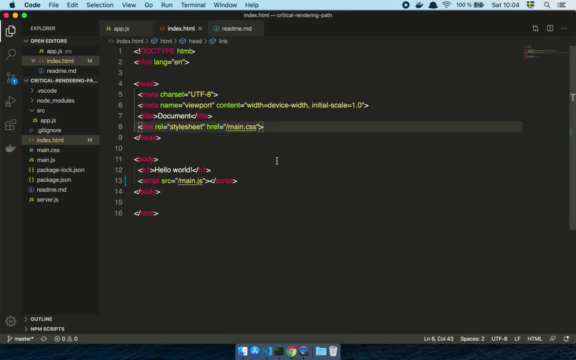 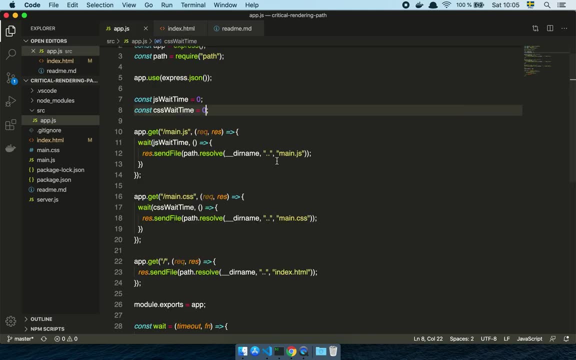 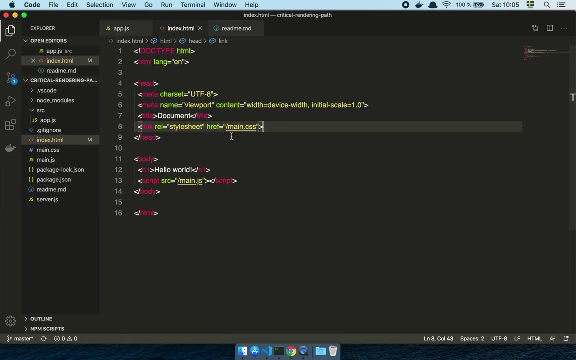 the better, because if one of them is really really slow, then you're going to have to wait for that one. it's better to have a one file than 10 files to get. it's going to be much more performant in general. of course, right scripts are also blocking, so if we have a look here, you'll notice. 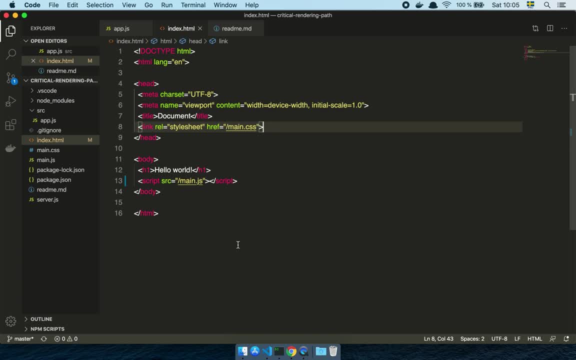 that i have added my script tag here at the bottom. this page here should be feel very familiar to you if you're doing any type of development work on the web. so what i could do here is that i could do something like this and this. you shouldn't be doing this. there are situations where you 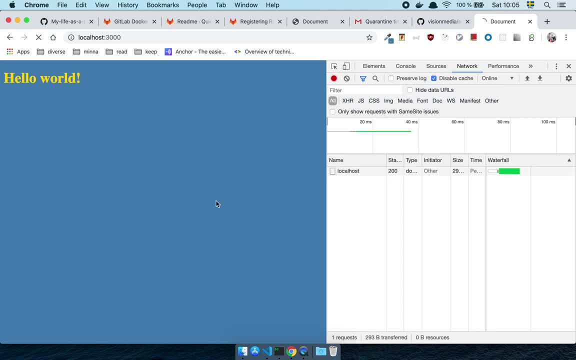 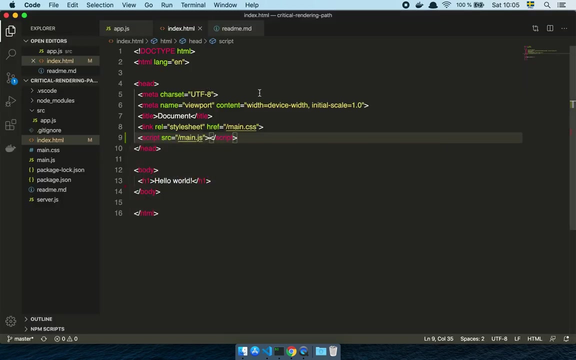 could be doing this, but if i do this, you'll notice something, and that is that i see the hello world check this alert before i see the text, because the exact same thing is happening. so alert is a blocking operation, but the script is also blocking, so what's happening is that i'm hitting this line. 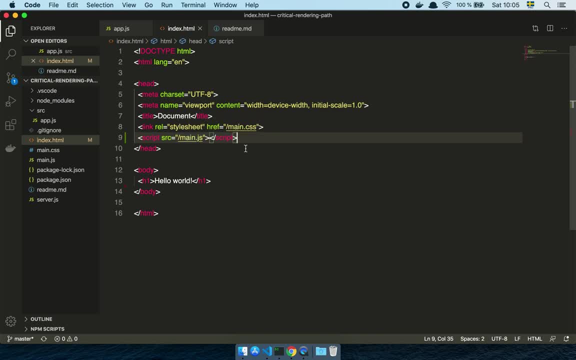 i'm getting my css file and then i hit this script. i get that script and then i'm executing, i'm going that script before the i'm going to continue, or the browser is going to do that. so this line here never runs until this thing here is resolved. so that's another thing to make be aware of. 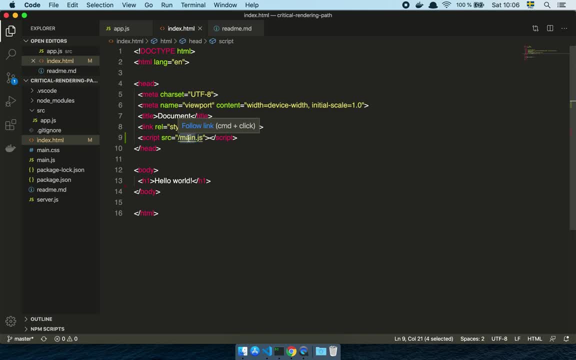 that if you have javascript and unless you need it to run before the dom is actually rendered out, which is, we will touch on that as well. there are situations when you want this. most of the time you don't want that. most of the time you want to have this thing here somewhere out, like at the at. 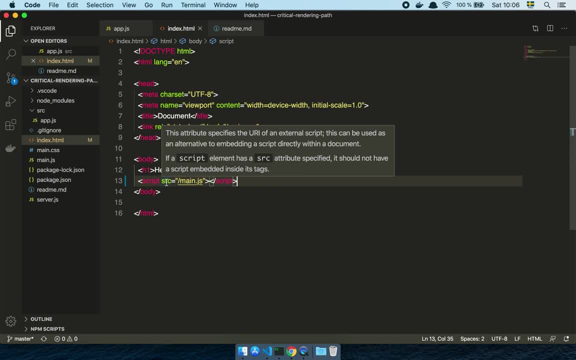 the end of everything. it should not be. you can put it outside of the body as well, but whatever you do, don't put it at the in the head, because it's going to run all that code before the user sees anything and if you have, you know, a really big library of a lot of complicated 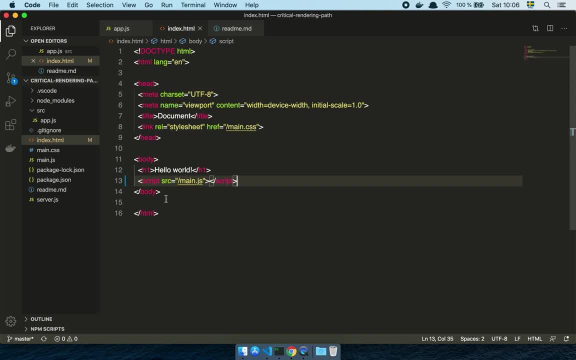 javascript: a big, big javascript file that's going to pretty much not render out anything onto the page until that is resolved. now there is a a special case as well. like you have to remember, this is for html, like what that we're sending from the server. if you're using an spa. 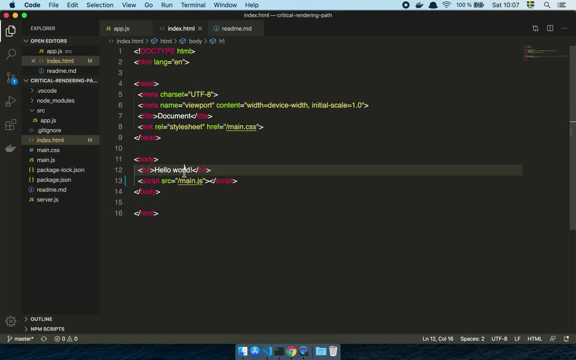 such as react or angular review. it's different, because then you're not not actually sending the raw html over the wire like this. what you're actually doing is that you're sending javascript and then, when the javascript loads, it will render all of these html elements to your page. so just 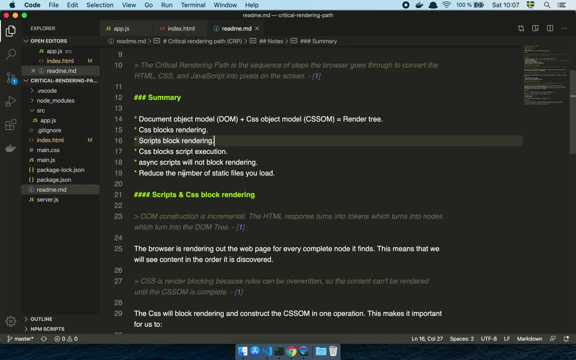 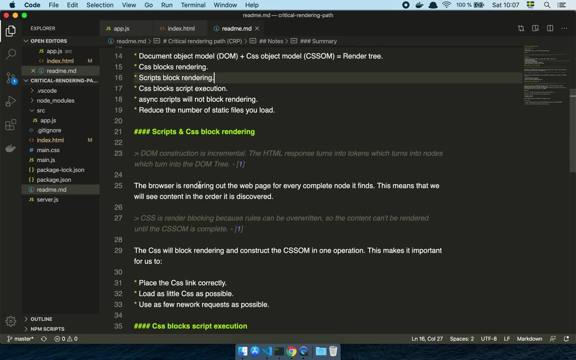 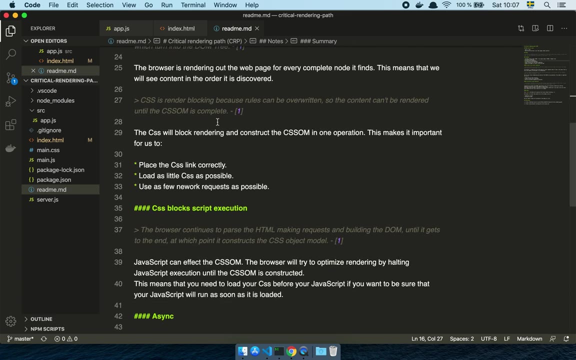 make sure that you understand the difference there. this is true, this, this rendering, is only true for the javascript you're actually sending html. so another thing to know about is that css- as we were talking about this definition here, the scripts and the css are going to block rendering. 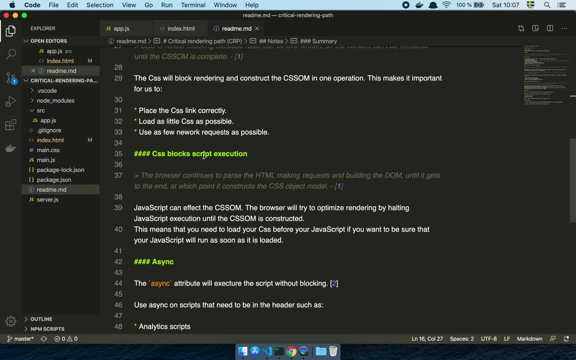 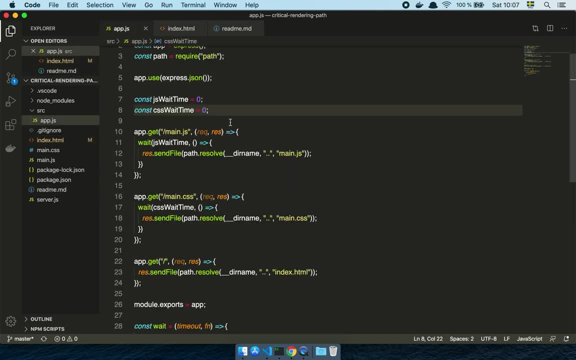 but there's something that is also worth knowing, which is that css blocks script execution. this is very interesting. so if i do something like let's say that i'd go back here and i say 10 css wait time and then i say, no, actually, let's do do it like that. we don't have to do it that way. 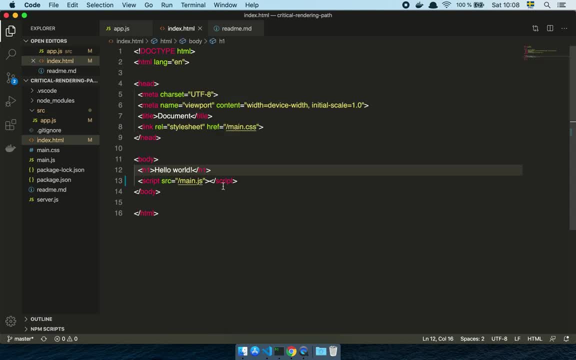 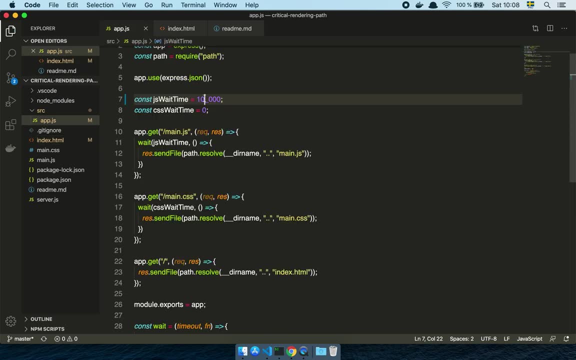 10 000, so a really, really slow javascript fetch here. let's do that now. what am i doing? it's supposed to be like that. here we are. so now, what i've decided is that, okay, we're going to have a javascript file that is fetched. 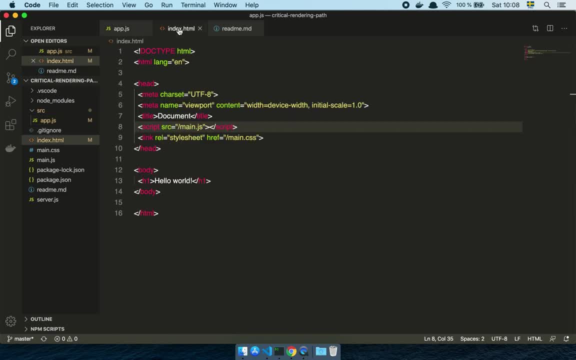 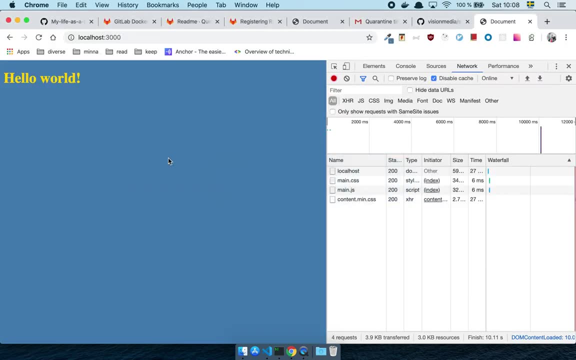 immediately, and then we're going to have a really slow network call to the css and notice what i did here. so now i put my script tag before my css. look what ha looks. look what happens now. so now this javascript is executing even though the css isn't done, which is fine. but if i reverse it? 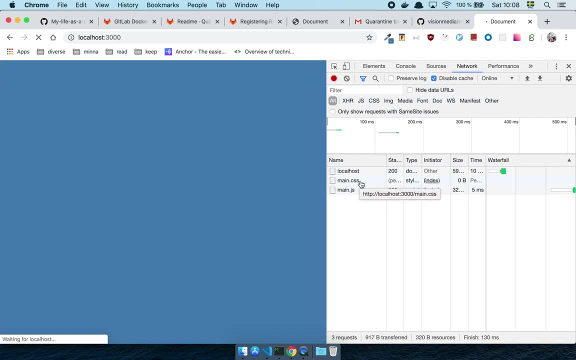 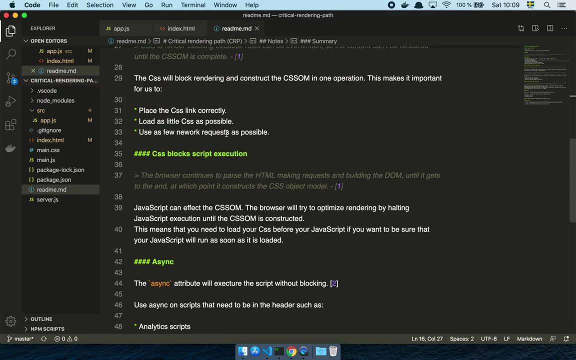 notice that nothing is happening. the javascript file is loaded, but the css is not done, so the javascript is now waiting for the css to come in. and there it comes in. and there you see my alert box. now what's going on with that? well, as i was saying earlier, this has to do with how the css object module is constructed, the 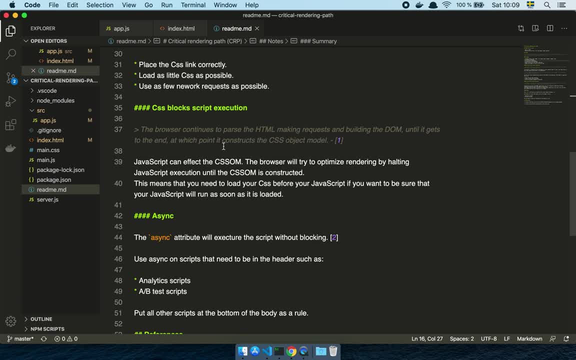 javascript. since the css object model is, it's possible for javascript to change the styling of the page, the browser will basically block the css object module and the css object module will be blocked until the css is resolved so that it is safe to execute the javascript. now you can override. 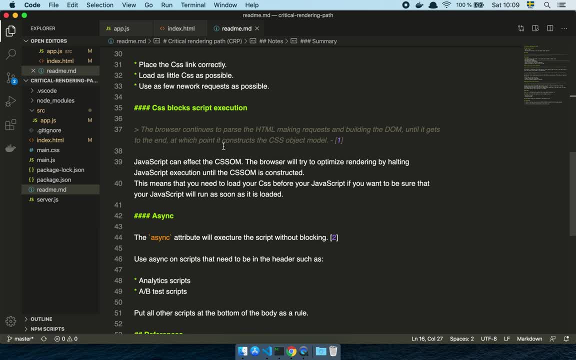 this and i'll show you how to do this, but that is the default behavior, so that the browser can be certain that, oh, i have all the css on the page now. now it's safe to execute that javascript, because that's the javascript might be changing something like class names or styles and things. 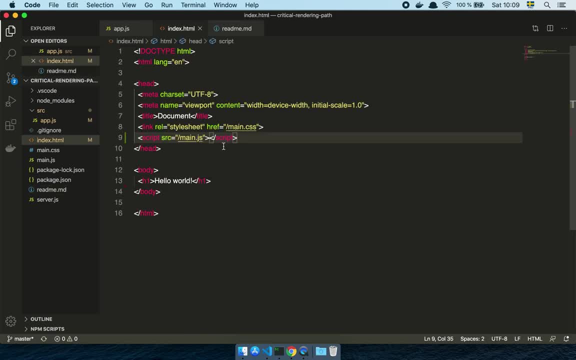 like that. so what you should really take away from that is that it's very important in general terms that you make sure that if you're, if you want something to run as like a javascript or something like that to run as quickly as humanly possible, it should be the first thing you do. but in general, 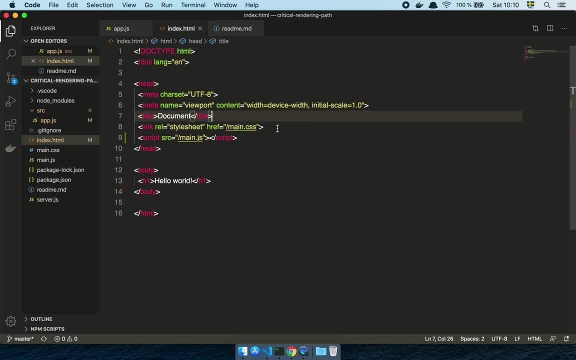 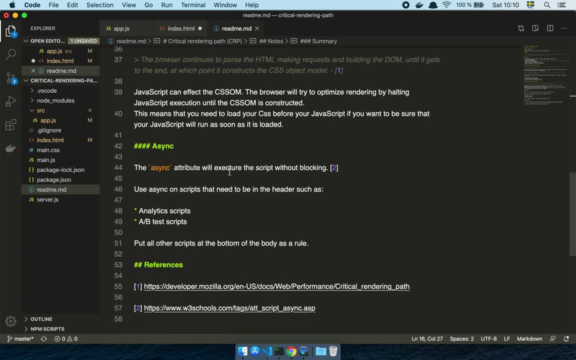 terms, what you want for is to make sure that the css is present before the javascript, because if, as i was saying, it will wait on with executing the javascript until the css has been resolved. so, finally, we can have a look at the async attribute. you can, and you might be familiar with the defer attribute as well. 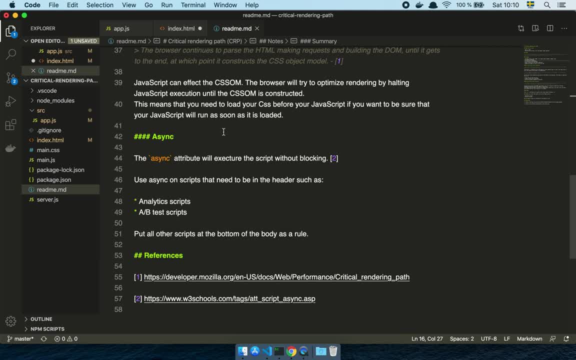 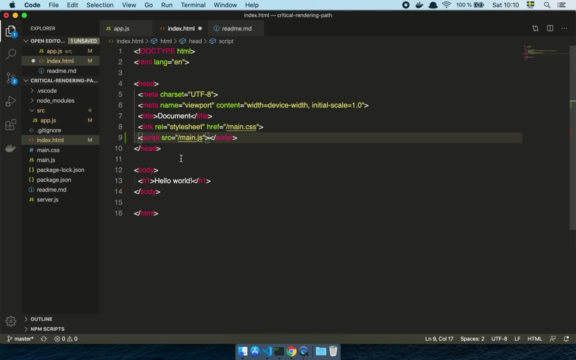 but i'm going to use async because it's a more common standard these days. so async basically means that i can override this behavior. i could say that: okay, well, i want the javascript here. it's still, it's going to load and it's going to stop. my hello. 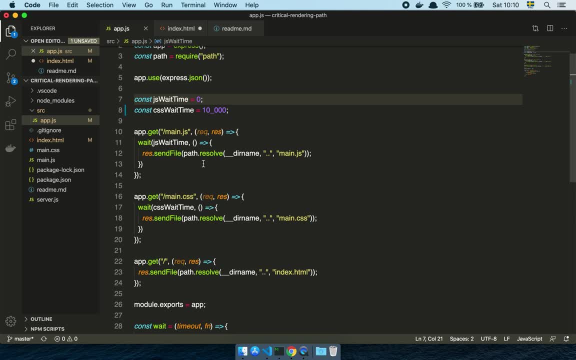 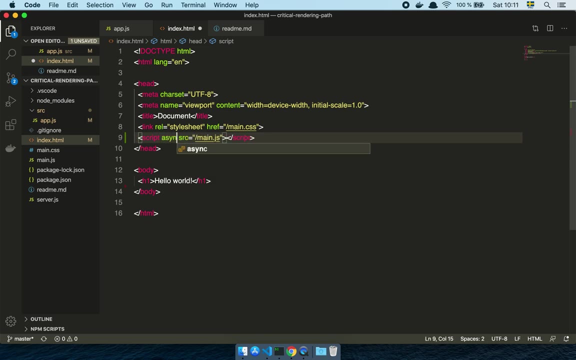 world tag here from being rendered, but i don't want it to take waste a lot of time doing that, because i know that i don't have to wait for this script to finish before i can render out the rest of the page. so what i want to do is that i want to say async. now, what this means is that this script 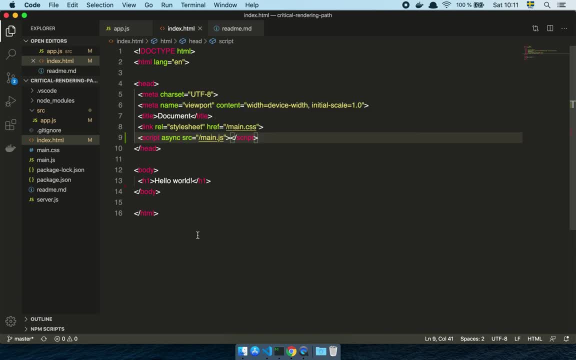 here is going to be loaded asynchronously to the page, so the browser is going to see this tag and go: oh, i see here that you made this an async script. okay, i will just fork that off into its own process or its own own thing and continue with my dom parsing. 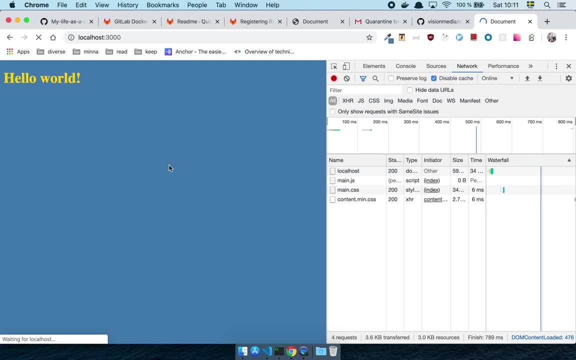 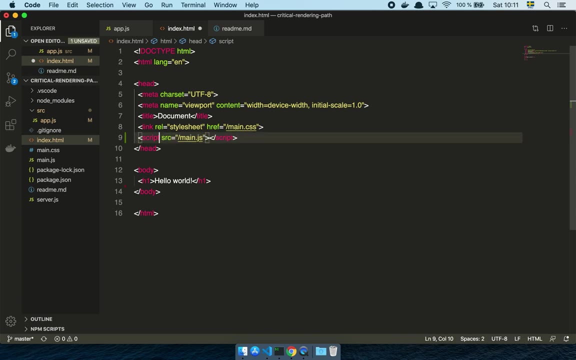 so now, even though notice that i refresh the page and i see my hello, the hello world text up here, even though the script isn't done, and as soon as it's done it's going to fire, there we are and this is a way for you to, because if you don't have that script, as we saw earlier, what's going? 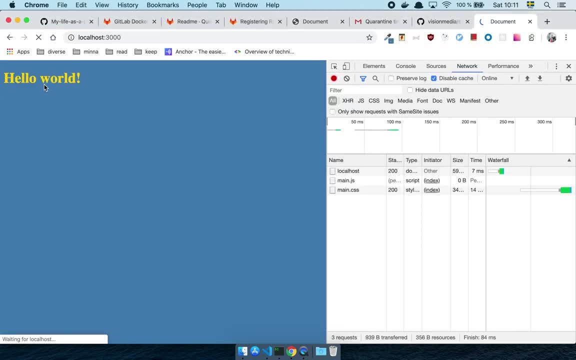 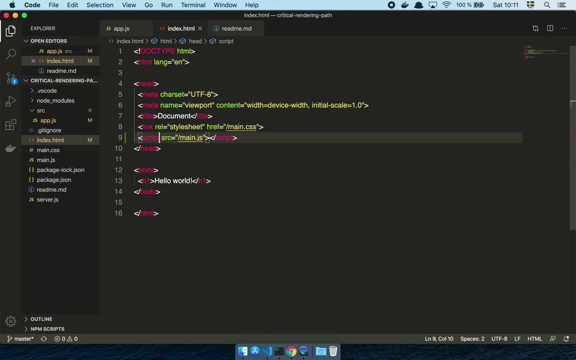 to happen is that it's going to as it takes a. the caching is still here, as you can see, it's it's not going to render out the html, even though i have the file. so with async you can override that behavior. cool, so that is pretty much all of these things. 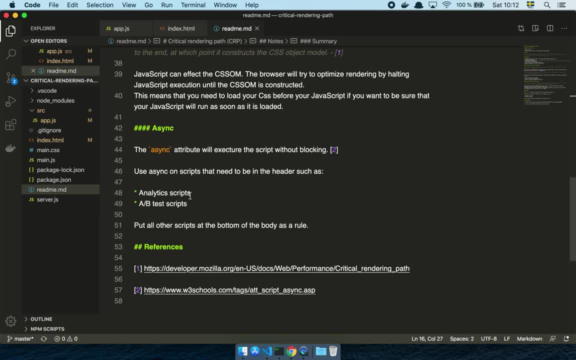 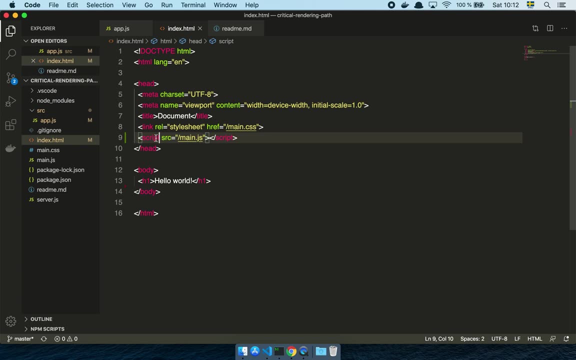 covered now. now, in general terms, the times you want to have a script in the head and maybe you want to do it in an async fashion or something like that it is. it's usually when you're running analytics or if you're doing a b testing or stuff like that. it's very rare, i mean, if you're. 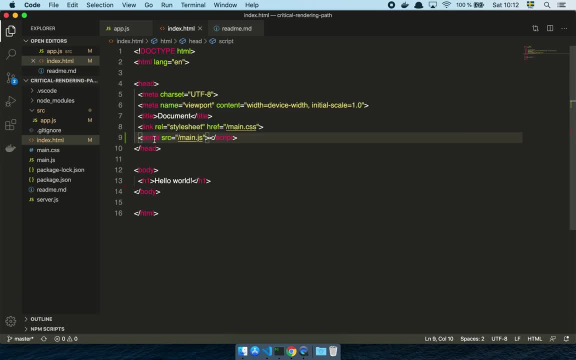 loading a react app or something like that. this is not the place that you want to pay put this sort of stuff. you can make it async, of course, but just as a rule of thumb, always make sure that you keep your script be after all, the content that you want to be rendered out as quickly as possible, and then 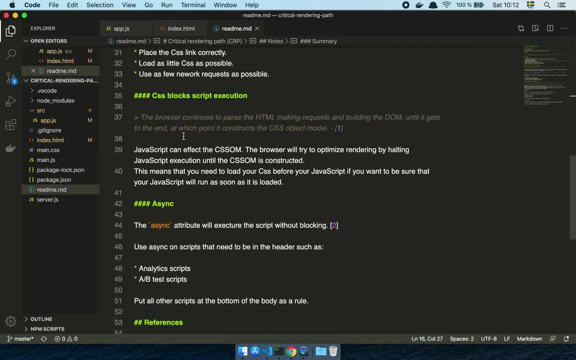 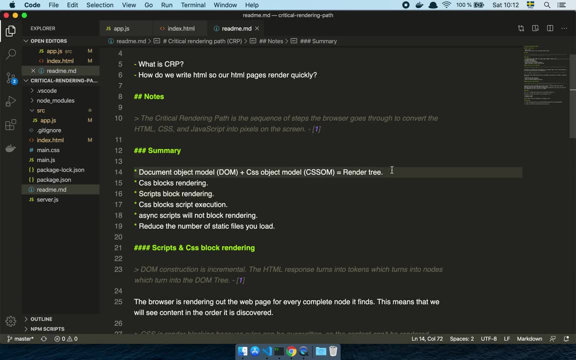 you should pretty much be fine. so what i want you to take away from this is basically this summary up here. so the dom and the css arm, or the document object model and the css object model is the thing that it creates the render tree, and that needs to be. that's the thing that the browser is going to. 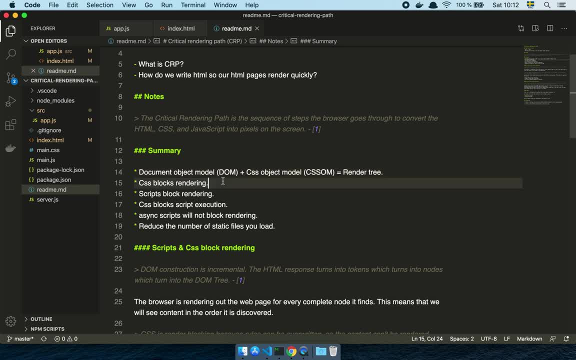 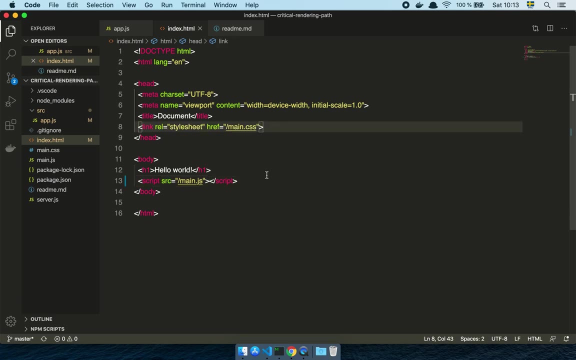 use in order to render out all those pixels to the screen. remember that css blocks rendering, which means that if you have a really big css file that you fetch, no, the user will not see anything of any of this html until that file is resolved. so if you want the fastest possible first render time, 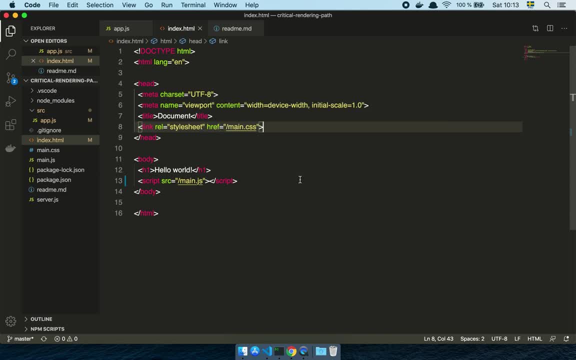 don't load css synchronously like this. you need to fork it off or wait until you like inline your styles or do things like maybe having above fold on your styles, or do things like maybe having above fold content, or there are many, many tricks that you can use in order to speed up that initial load. 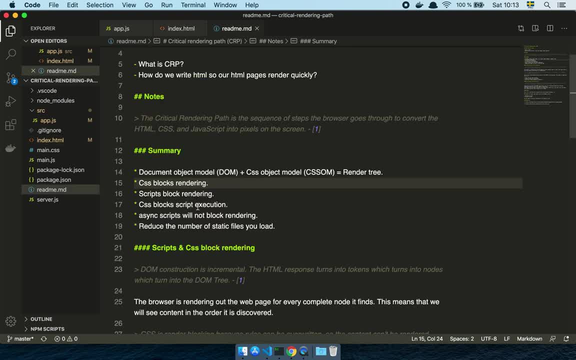 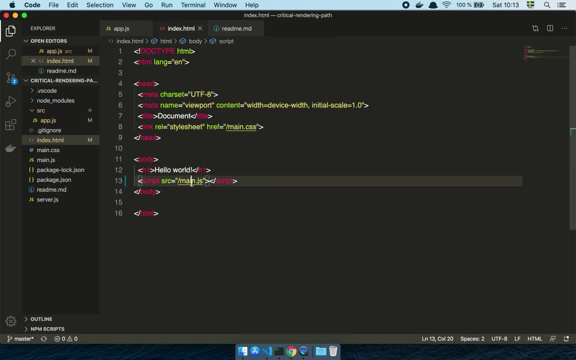 time or the first render. so that's that script block scripts blocks rendering as well, which is as we were saying: make sure that your script is the last thing that happens on the page, or that you, at the very least, make sure that you make it async or something like that, so that it doesn't. 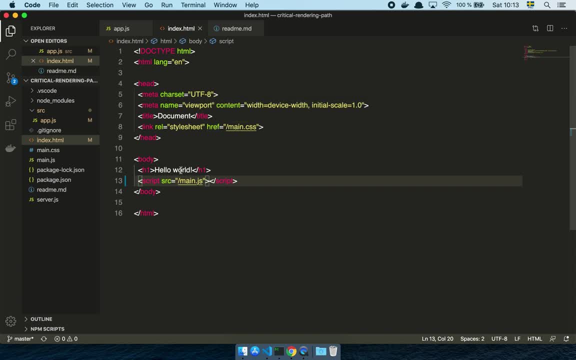 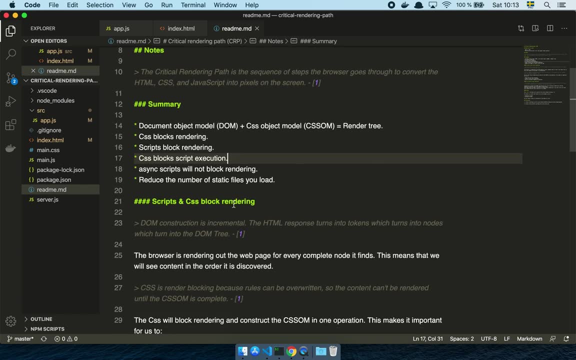 block in the head because it will not show any html to the user. if you do that, then you also need to remember that css blocks script execution. so if you have a really large amount of css and a script that needs to run and you want that script to run as quickly as possible, 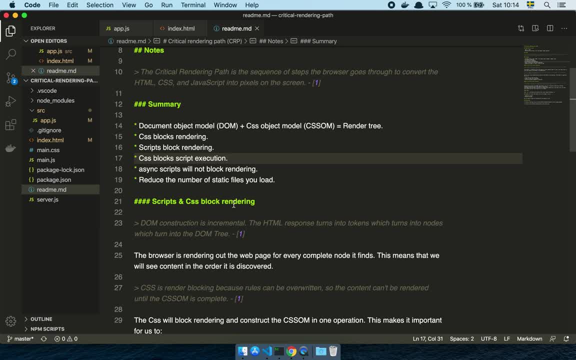 you need to make sure that that script isn't being blocked by the css, because it will hold that execution. if you add async to the script, it will. it will basically just run in parallel to the, to the works or asynchronously to the page renderer. so you can basically be sure that the 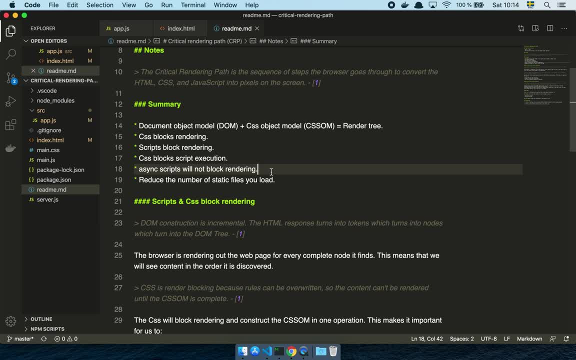 script will run whenever it's done. it doesn't care about the remain, the rest of the page. and the best tip i can give you for having a good crp is to reduce the number of static static files that you load. it's better for you to have one big file than have many small files. 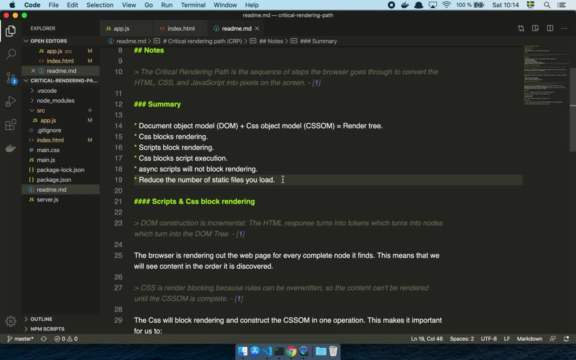 because, as we were saying, the more network calls you make, every network call is going to stop the browser and every time you make a network call, odds are that it there will be a delay on the internet or the wire is going to be funky in some fashion. so, with a 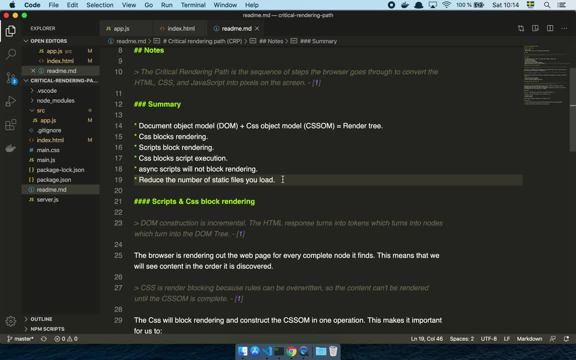 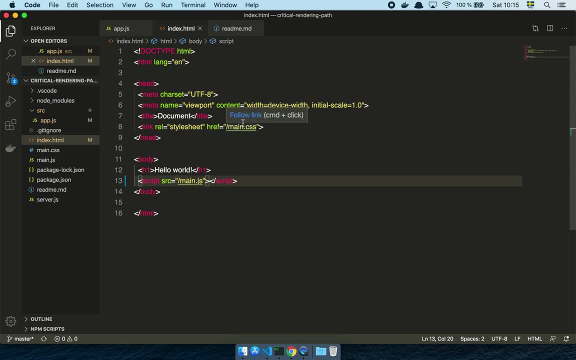 bigger file. odds are that you will get all that data to the user quicker. and, apart from that, make sure that if you're really interested in making sure that your your page loads as quickly as possible, just use standard html and inline styles, because then it will load as quickly as it can. possibly load. have a great day.